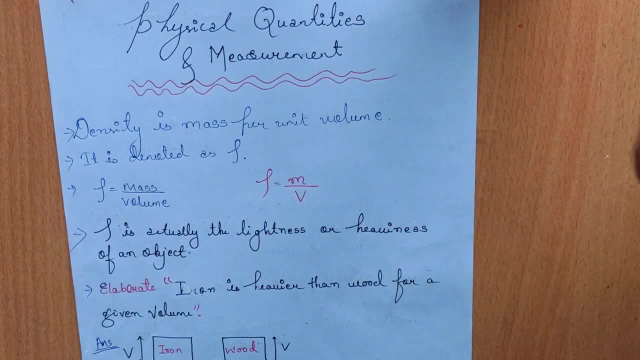 What is the name of the chapter? Physical Quantity. So you should know the meaning of Physical Quantity. So Physical Quantity means that quantity which can be measured. So here we will study about those quantities which we can measure. And measurement means, you know, measurement means like measurement, okay, 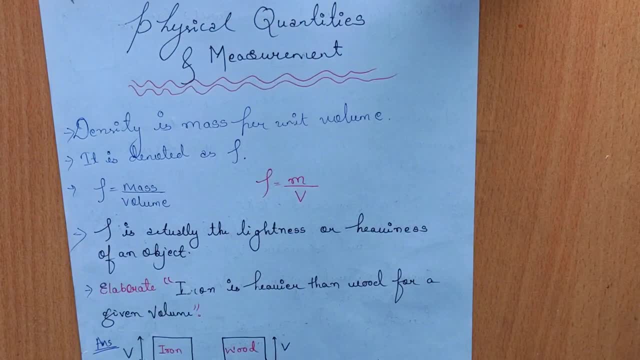 We measure an unknown thing with a known thing. That is called measurement. It has a different definition, but I am telling you in a normal way. Okay, So here, like children, in the intro in the book basically it is given about density. 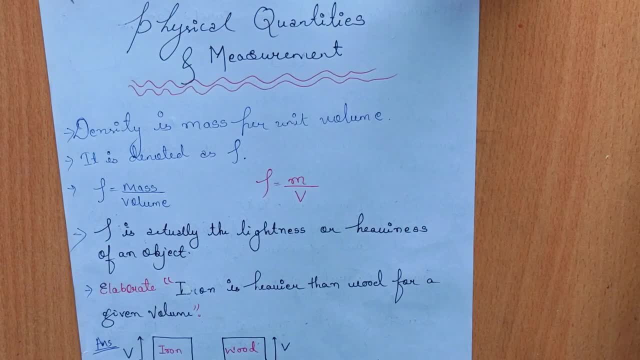 And in this chapter it is given about things related to density only. So we also start with density only. So what is density? children See like we say something is light or something is heavy, Light and heavy. So that is actually related to density. okay, 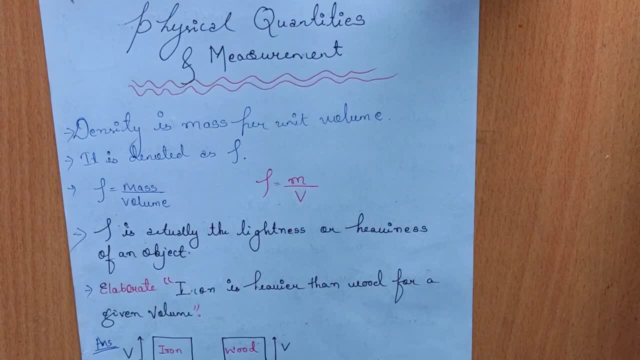 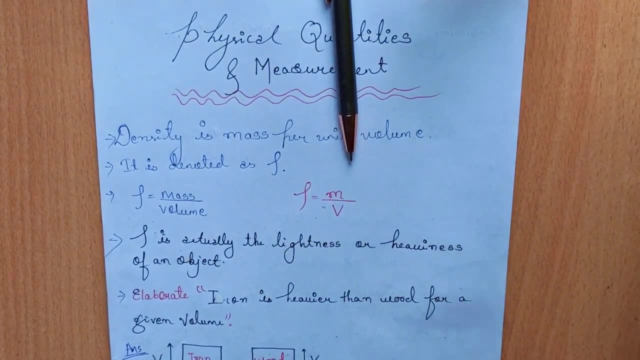 That is actually related to density. Till now in class 6 and class 7, what did you study about density? What did you study about density? So density can be defined as mass per unit volume. We can define density like this: 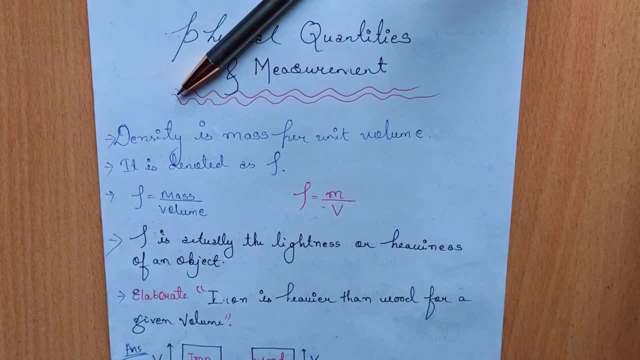 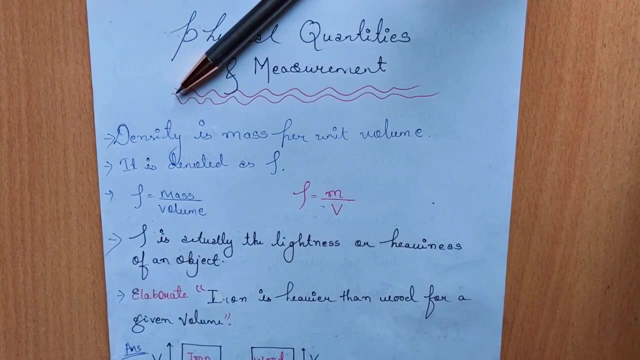 It is a very simple definition: Mass per unit, volume. This per unit means basically divided by Or. you can see in its expression, or in its mathematical expression: Density is equal to mass by volume. Now, instead of density, I have written here rho. 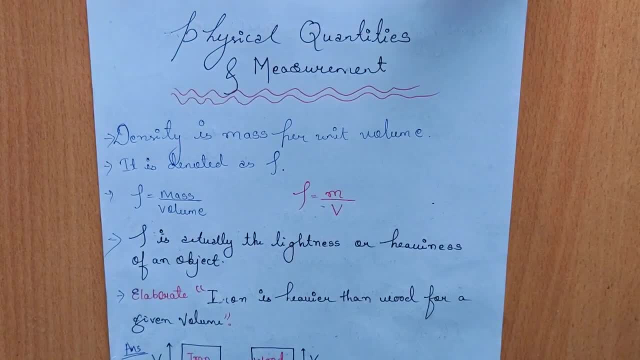 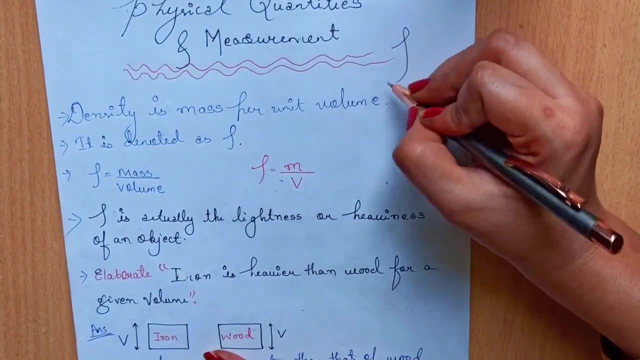 Here a symbol will be seen. It is written somewhere, pico. So here it is rho. Okay, This is rho. How will we write this? I will write it once and tell you. We normally make it like this, Okay. 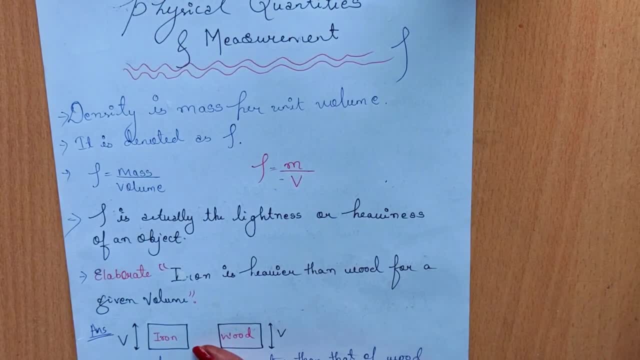 So this is rho. Instead of density we write this, And the formula of density is always written Mass by volume. In higher classes there are different formulas of density. You will read that, But for now you have to remember. 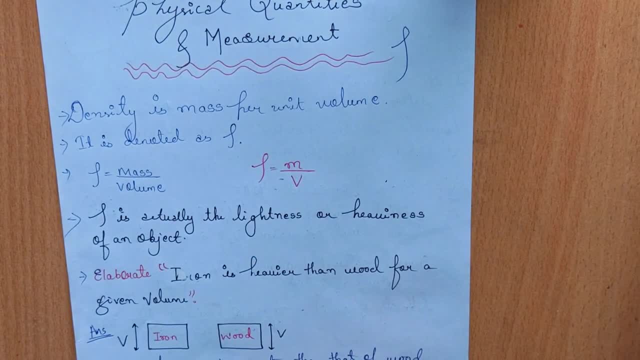 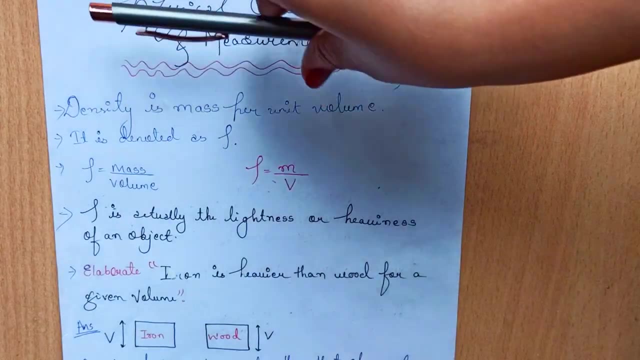 Density is equal to mass by volume. That means density is related to mass And object is related to volume. Both are related. So you can take any object. You can consider this pen, You can consider this paper, You can consider this table. 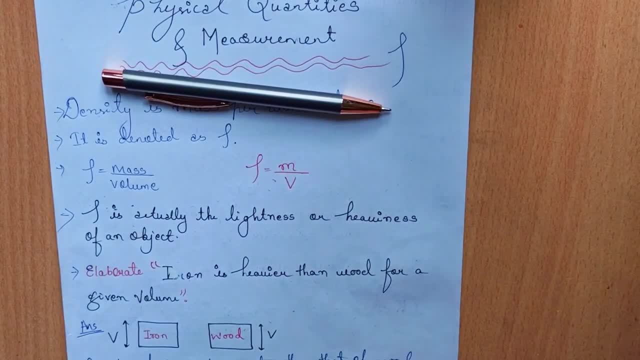 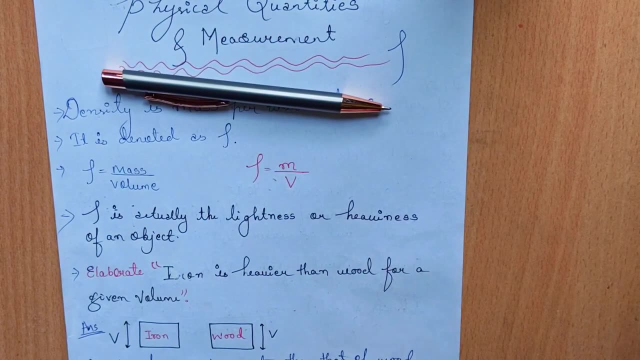 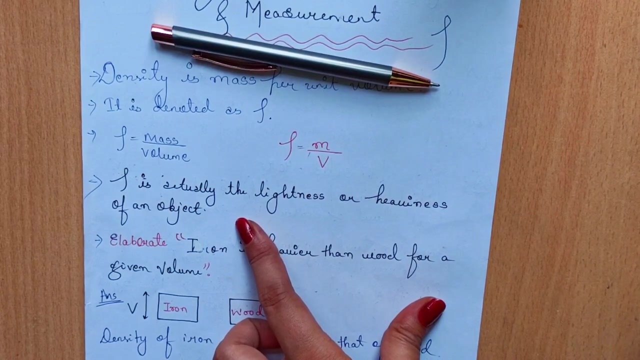 You can consider anything. Whenever we define density or consider it, We will keep in mind the mass and volume of that object. So density is actually the lightness and heaviness of an object In simple language, if I talk. How to understand it in a simple way? 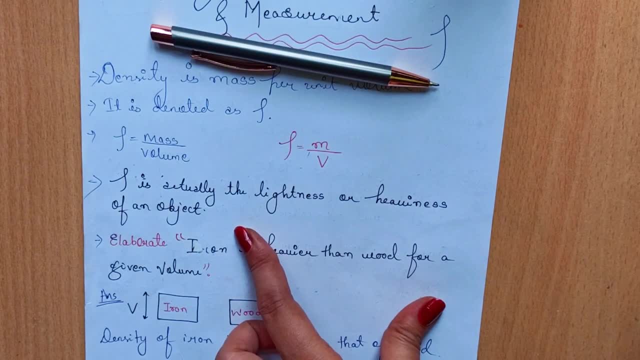 It is actually the lightness and heaviness of an object. It is actually the lightness and heaviness of an object. It is actually the lightness and heaviness of an object. We can understand it in a simple way. Now there is a statement here. 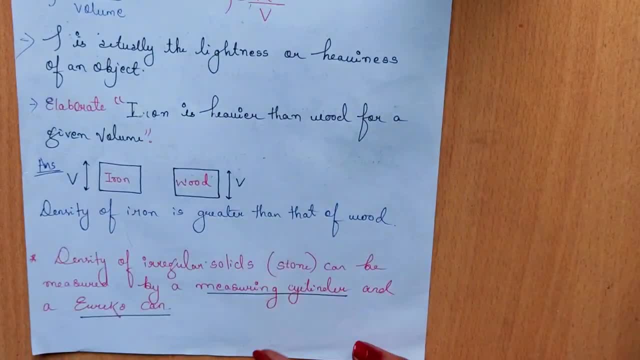 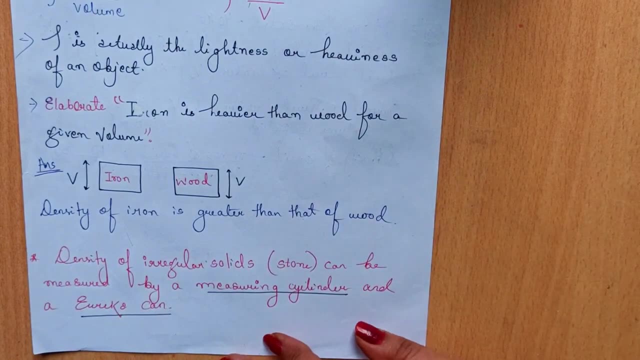 You can see a line here. Iron is heavier than wood for a given volume. Suppose you have two things: One, you have, iron. Suppose you have- I have already made the diagram. Suppose you have a piece of iron. 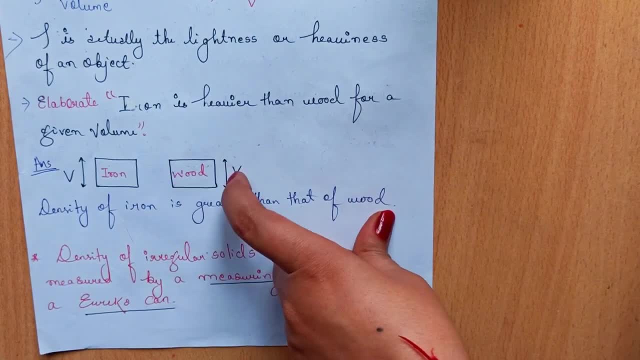 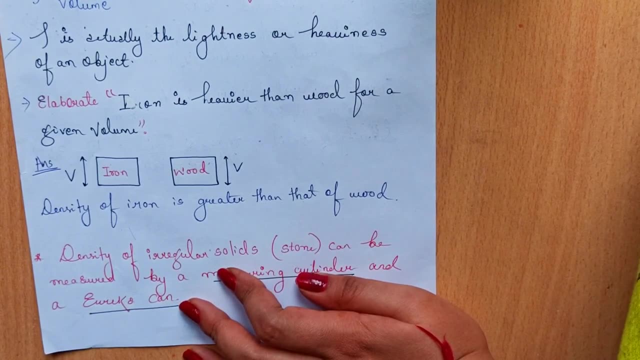 And here is a piece of wood And both have the same volume. Given volume means Suppose both have the same volume. Given volume, Then both have the same volume And when you measure the density of both Then you can see that. 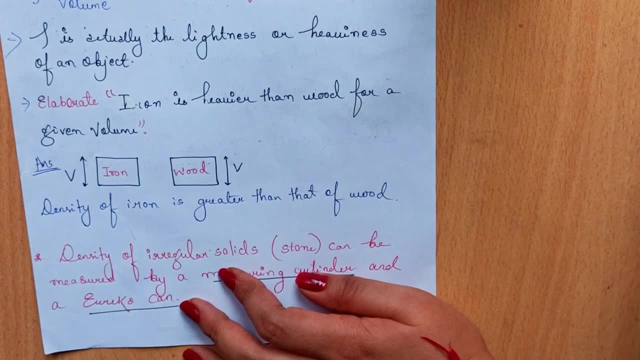 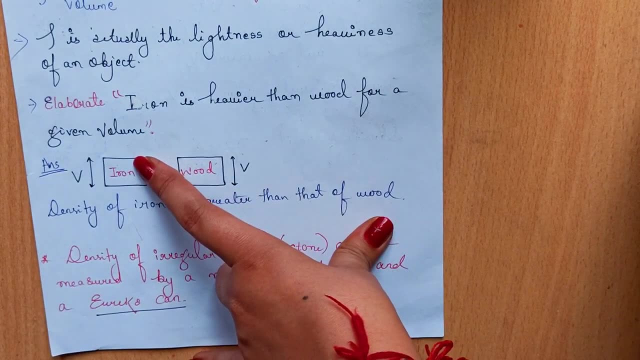 Iron is heavier than wood. Iron is heavier than wood. Iron is heavier than wood. It means that Density of iron is more than wood. Density of iron is more than wood And mass of iron is higher than wood And mass of iron is higher than wood. 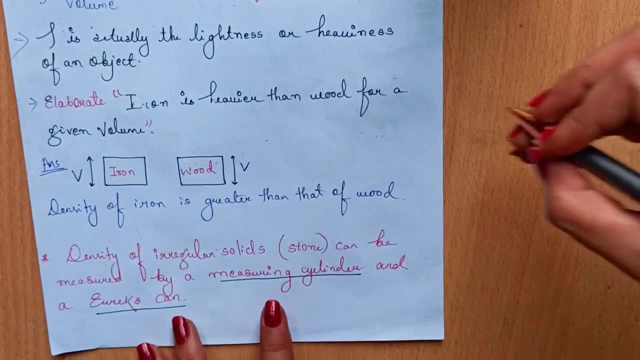 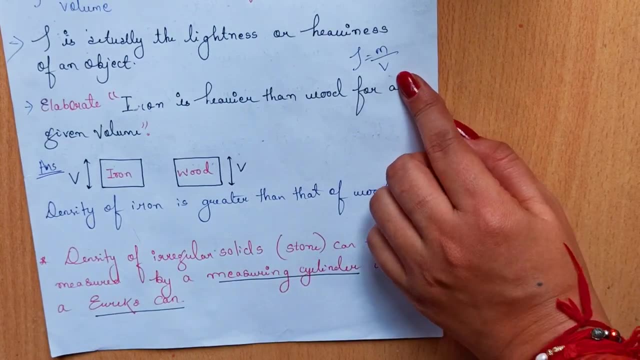 How is mass more than wood? If you look at the formula- I am writing a formula here- Mass by volume, Volume to dono ka same kar diya gaya hai. The volume is the same for both, Aur bol diya hai ki bhaari kaun hai. 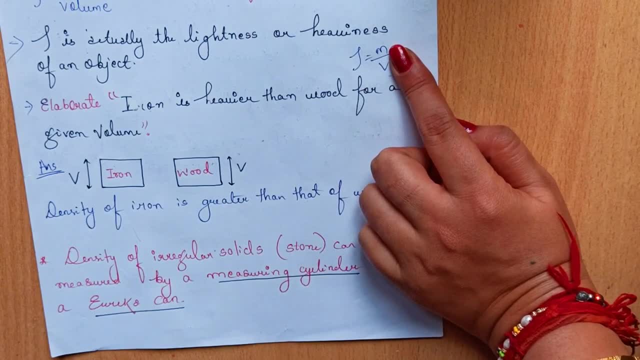 Iron bhaari hai. Agar volume same hai, to kya baj gaya mass? Agar iron is heavier, That means mass of iron should be heavier than wood. To yaha par aap loong ko is type se likhna hai. 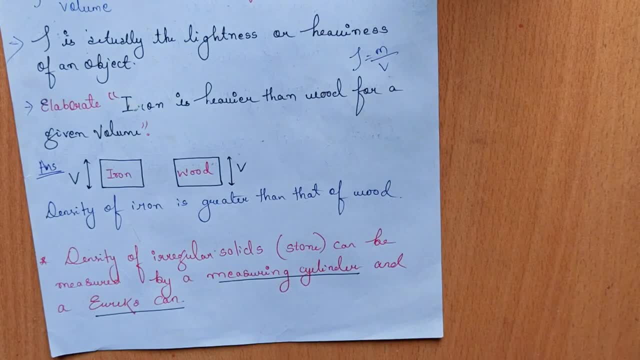 Exam mein, agar aata hai, Elaborate karo. Ya bas one mark ka teacher push dete To aap loong is type se like kar sakte ho, Bata sakte ho, Explain kar sakte ho. Baht simple hai. 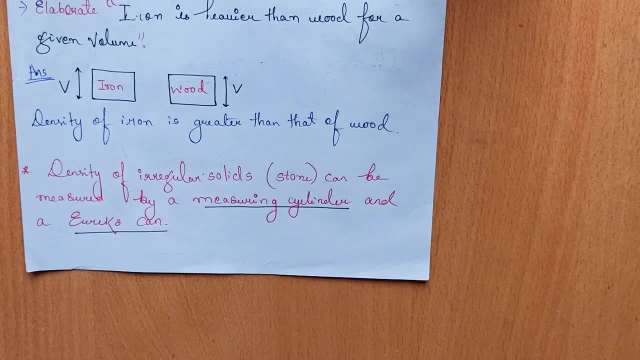 Thek hai Now Abhi Ha, Ab dekho, bacho Ab desi, ki bahut saare alag, alag type ke naa substance hota hai. To hum loong alag, alag type ke substance ka density ko measure kar sakte hai. 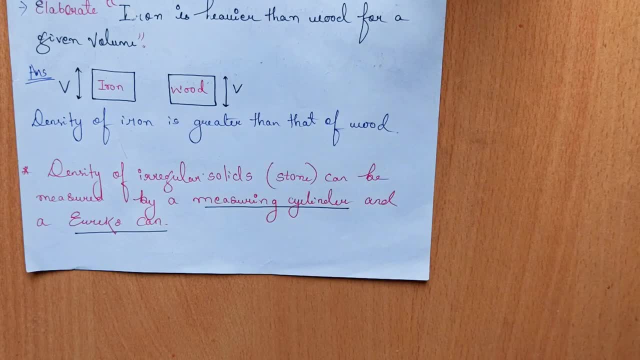 Yaha par mainly solids ka baat ho raha hai. Thek hai, Koi bhi hard chee solids ka baat ho raha hai. Aap sab ko pata hai, solids kis ko bolte hai. To agar mai baat karoon ki koi irregular solid hai. 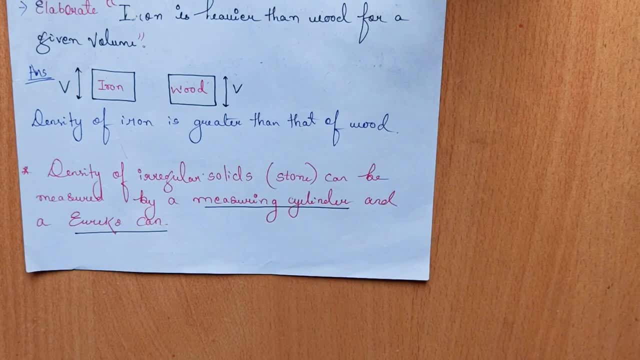 Irregular solid matlab, aisa solid, jis ka koi particular shape nahi hai. Desi ki aap loong best example le loo: a piece of stone Thek hai. Ek stone le loo, Pathar le loo. 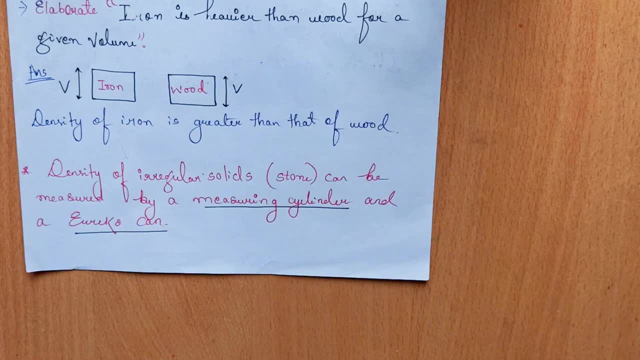 Aap loong rock le loo, Chalo stone le loo Thek hai To agar mai uska density naapna chaahoon To usko mai kaise measure kar sakti hoon To question aata hai bacho. 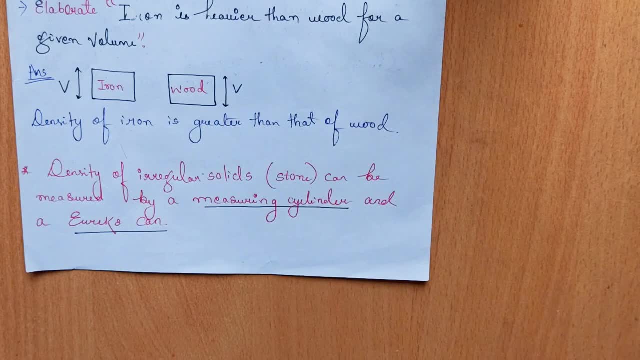 Ki how can we measure the density of an irregular solids Matlab? irregular solids ka density hum loong kaise measure kar sakte hai. So irregular solids ka density measure karne ke liye naa Do cheez aati hai, Ek hota hai measuring cylinder. 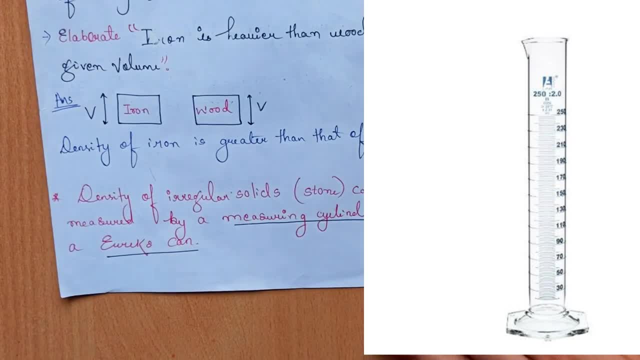 Jo ki aap loong book me bhi dikh raha ho, ka Said me maa diagrams de di hoon, Like side mea photo me de di hoon. Aap loong usko bhi dekh sakti hoon. 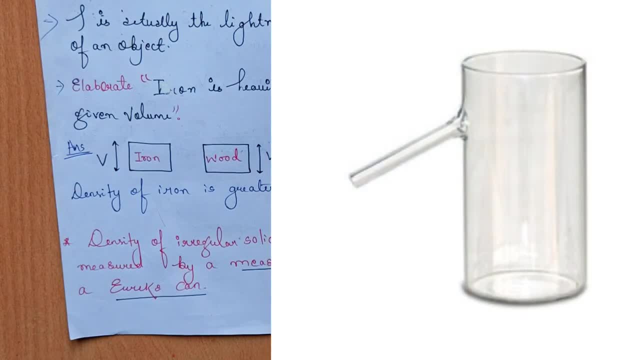 And second, hota hai: Eureka can, Eureka can bhi book me Like Ache se mentioned hai, Aap side me bhi aap loong ko dekhne ko mil raha hai, To yeh do cheez hota hai. 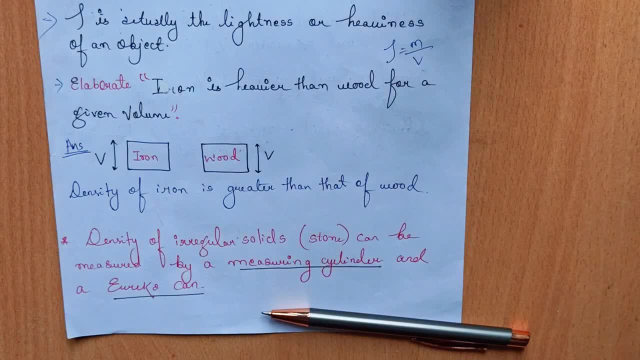 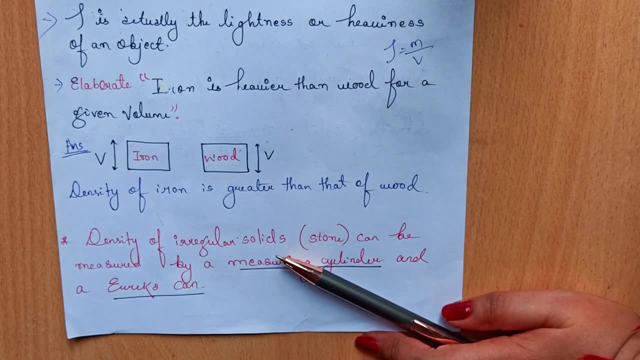 Usko use karke naa. Hum loong araam se bohot easily, Without any problem. Hum loong lab me Ya ghar bete, bete Ghar me kya Lab me hi? basically, Because lab me hi sab rehta hai naa. 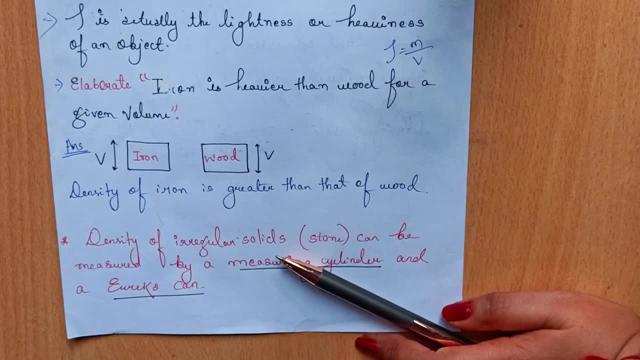 Samaan. So lab me hum loong araam se density irregular solids ka measure kar sakti hai. Ok, So do cheez ka naam yaad rakhna hai. First is measuring cylinder, Second one is Eureka can. 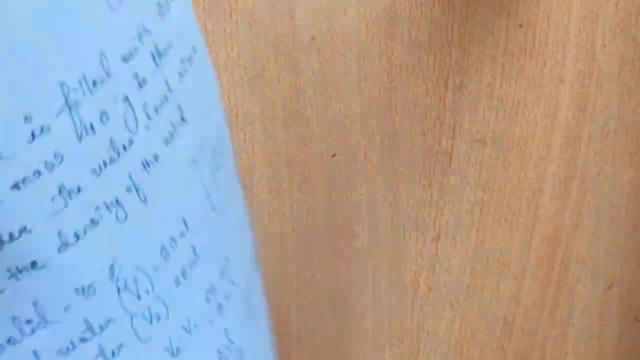 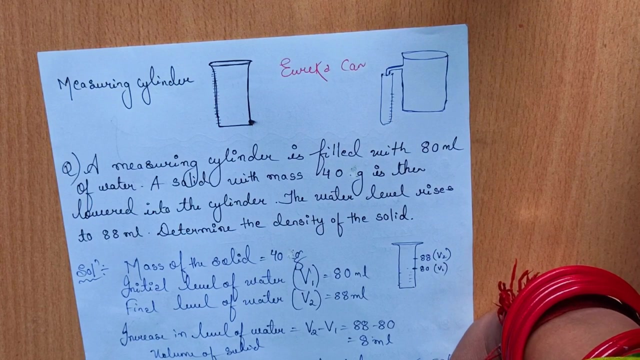 First is measuring cylinder And second one is Eureka can Ok. Aur yaha par bhi main diagram apne hesaap se like, jo mujhe samajh me aaya bana di hoon. First is measuring cylinder. Joki, aap loong dekhe ho. 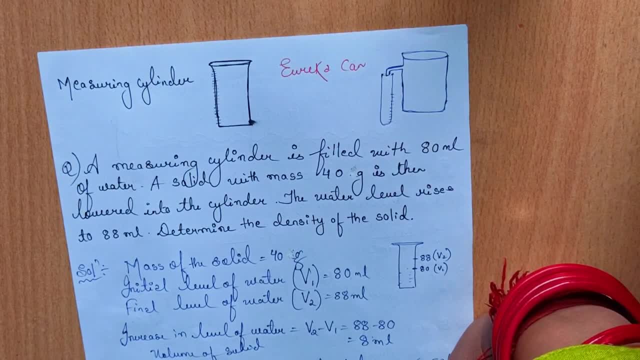 Alag alag shapes, me Alag alag material ka Like glass and basically plastic. Yeh do type ka material ka, Yeh available hota hai. Lab me bhi rehta hai, Plastic ke bhi rehta hai. measuring cylinder. 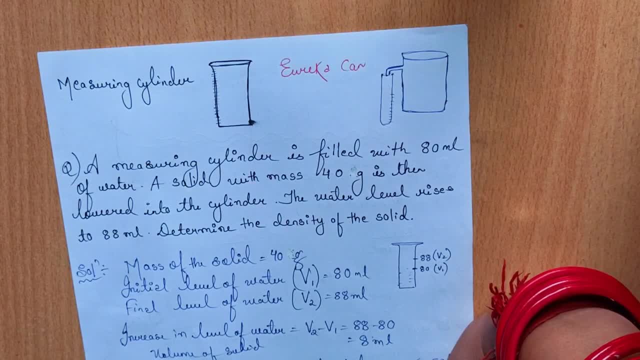 And glass ka bhi rehta hai, Thik hai. And isme naa yeh matlab graduated, Graduated rehta hai. Matlab iska matlab hota hai. Yaha par naa se scale bana rehta hai, Scale ka matlab hota hai. 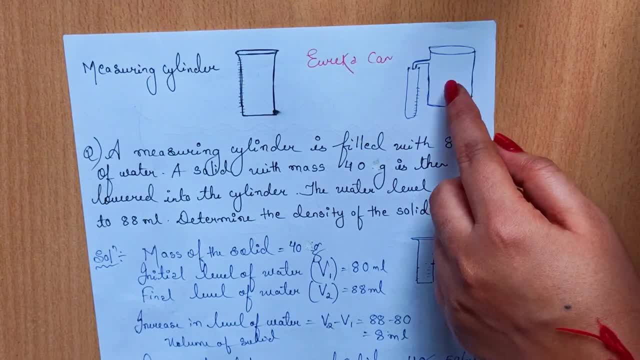 Maha par isme numbering rehta hai. Ok, Measurement ke liye. Aur yeh hai, Eureka can. Ok, Is type ka beaker rehta hai, Yaha se is type ka sprout rehta hai, Aur hum loong araam se measure kar sakti hai. 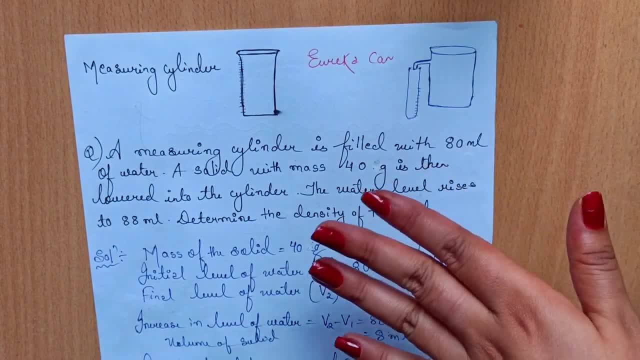 To isko hum loong use kar ke araam se like density, irregular solids ka measure kar sakti hai. Abhi, bacho, dekho me ek activity hai. Main to yaha philal nahi kar sakti ho. 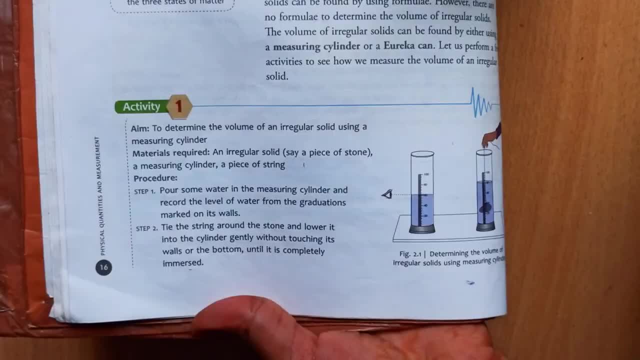 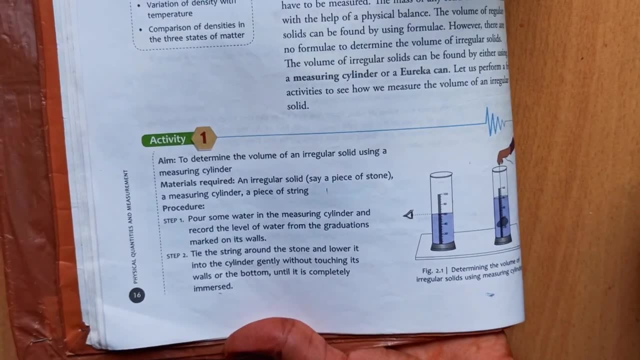 To main book ke through hi aap loong ko samjha rahi hoon. So yaha par hum loong ko Konal Ke activity diya gaya hai To determine the volume of irregular solids using a measuring cylinder. 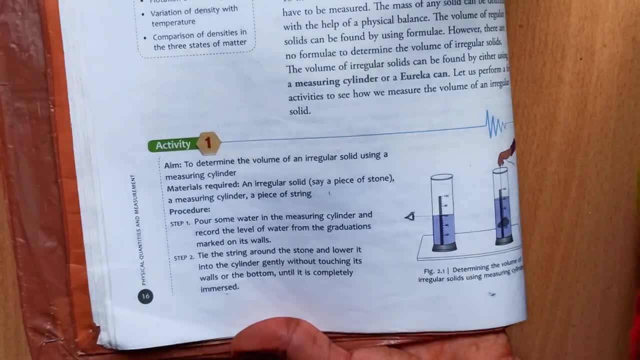 Measuring cylinder ko use kar, ke hum loong ko volume batana hai. Kiska irregular solids Matlab ek pathar le loo aap loong Irregular hota hai. Aisa hai toh ki particular shape hota nahi hai. 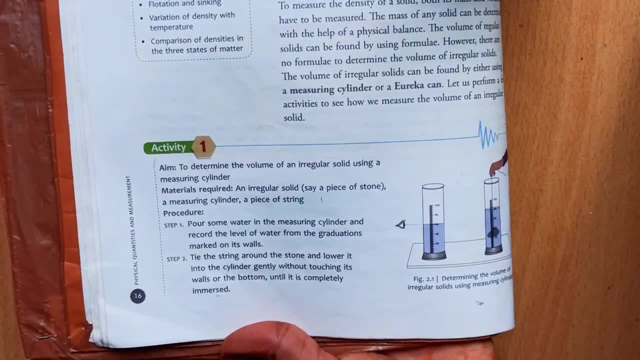 To hum loong ko naa usko volume dikhana hai, Like measure karna hai To bacho. yeh naa bahut easy hai, Like school me. toh kafi baar hum loong ne like dikhaya hai bacho ko. 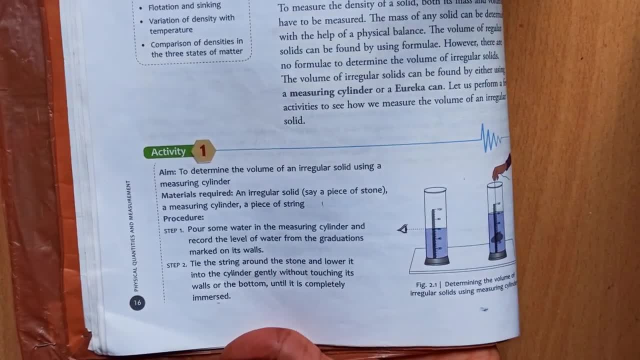 But abhi possible nahi hai. Wana dikha deti Main, agar mere paas samaan Available hota. Apparatus Tika To dekho, bacho yaha par. kya hai mainly Hum loong ko naa sabse pehle. 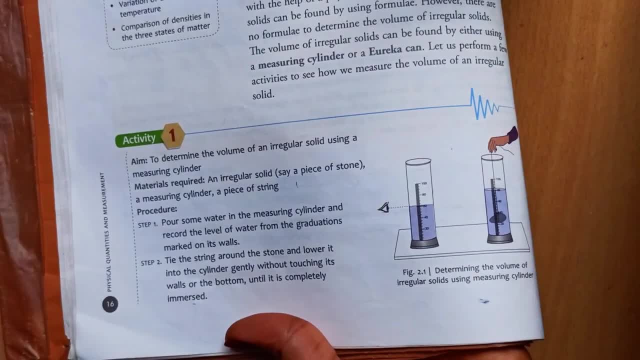 Dekho, yeh measuring cylinder chahiye, Ek chahiye. Tika Yaha par ek measuring cylinder le liya gaya hai. Ek aap loong aaraam se piece of rock, Rock, toh ni bolna chahiye. 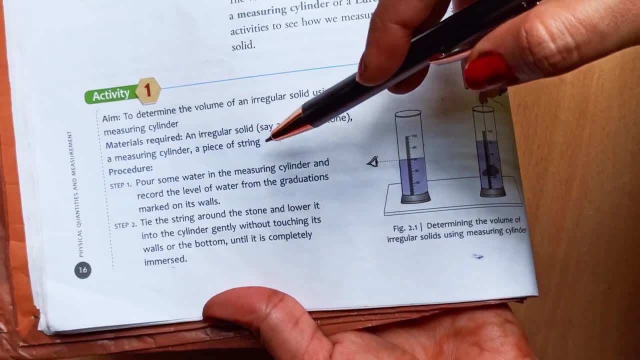 Stone, Stone le le naa, Measuring cylinder le le naa. Piece of string Jasi ki dhaga hota hai naa. Aap loong go le sakte ho. Lab me ek tam achche se diya rata hai dhaga. 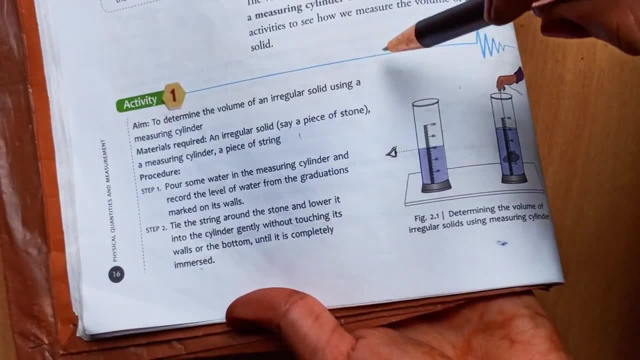 Tika string Hum loong ko yeh teen chis chahiye Toh hum loong kya karengi naa This is string. reyega Toh string se hum loong naa O pathar ko aise baand denge. 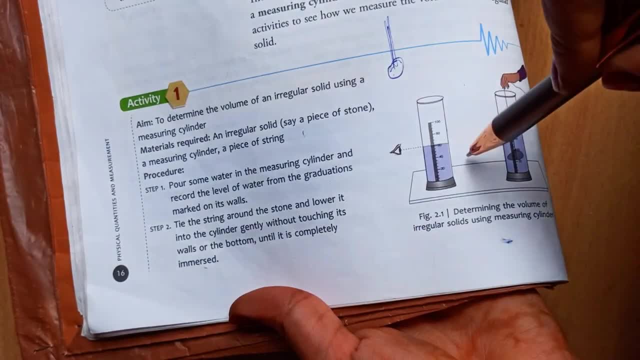 Tika O stone ko aise baand denge O yaha par measuring cylinder me naa Aise water le lege, Suppose Koi bhi level tak water le lo, Koi bhi level tak Jasi ki fifty tak le liya. 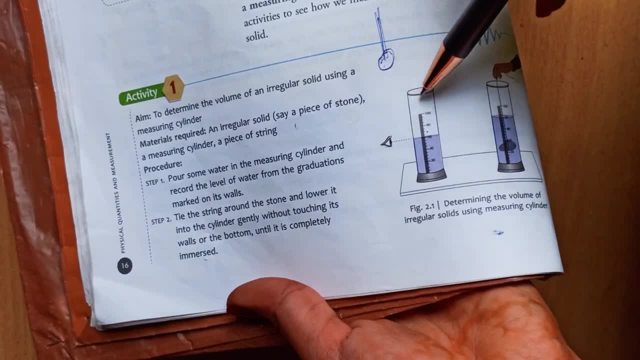 Yaha kitta le, ya Yaha bhi fifty tak le, ya Chalo Fifty tak le liya. Or jab bhi measure karoge naa, Toh apna jo eye ka level hota hai, O water ka level ke ekdum samaan. 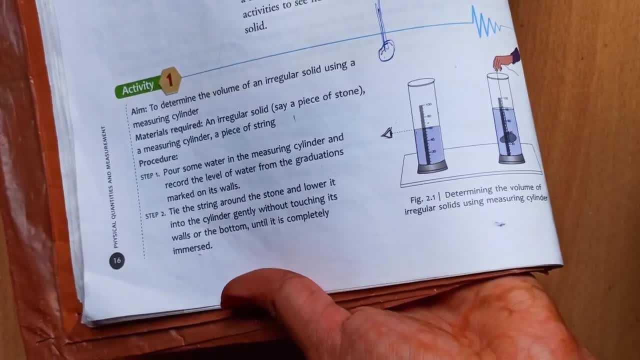 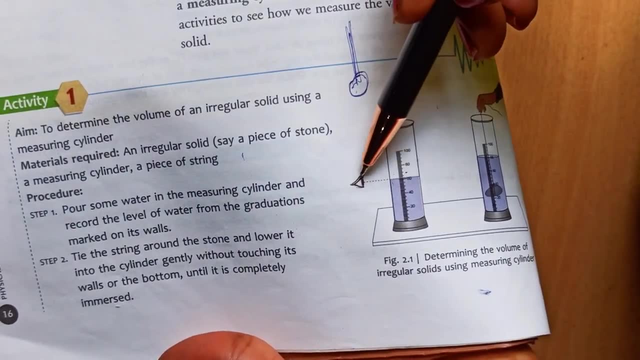 Ekdum seeda ho naa chahiye, Warna error a jaata hai. Lung ko toh itna pata hoga. Abhi tak toh Ki measurement hum jab bhi karte hai, Toh pura apna jo eye ka level hota hai naa. 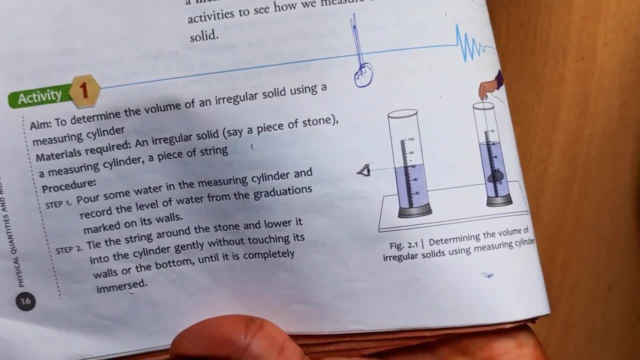 O water ka Ekdum level, Ekdum horizontal, Ekdum samane, samane ho naa chahiye, Tika, Toh ye aagaya. fifty Uske baad, hum loong, kya karengi. 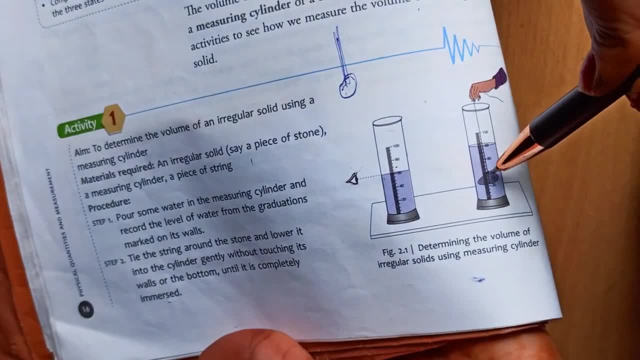 Jasi ki ye dekho string ko Joki attest hai, Kis se Stone se Usko ye kasi insert kar raha hai. Andar me Ye dhyan rakna hai Ki o side wood me touch naa ho. 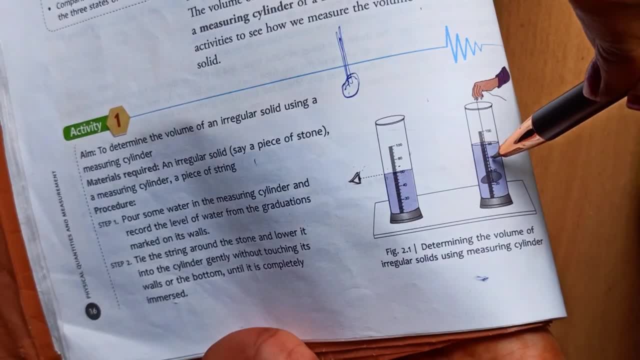 Ekdum seeda haplung usko dalna. Jab seeda dal doge, Toh aap loong dekho, hoge ki water ka level bad jayega Water ka level suppose bad ke ho gaya, Kitna ho gaya. 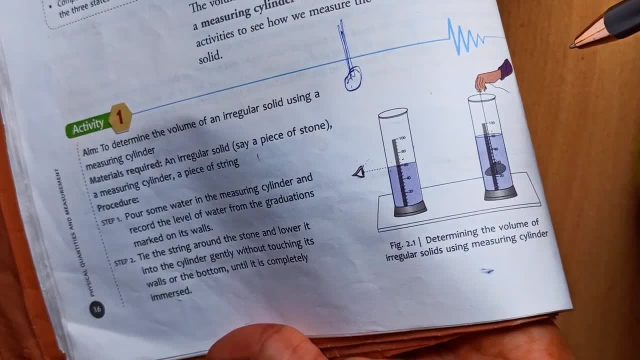 Sixty, Sixty ho gaya. Wo bhi aap loong measure kar loge, Tika Pahle tha fifty Bad ki kitna ho gaya. Sixty ho gaya Kitna increase hoa bacho. 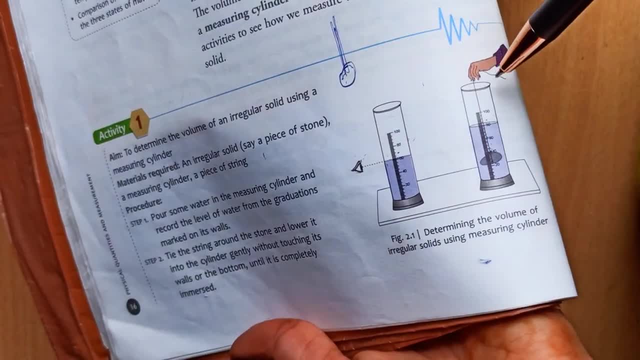 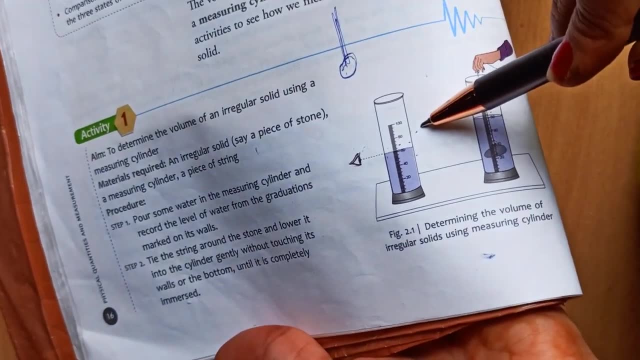 Sixty minus fifty Matlab initial tha pachas Bad ke ho gaya. sixty, Toh sixty minus fifty karna hai Final jitna hoa minus initial Initial matlab starting jo rehta hai: Tika Toh hum loong aise karengi. 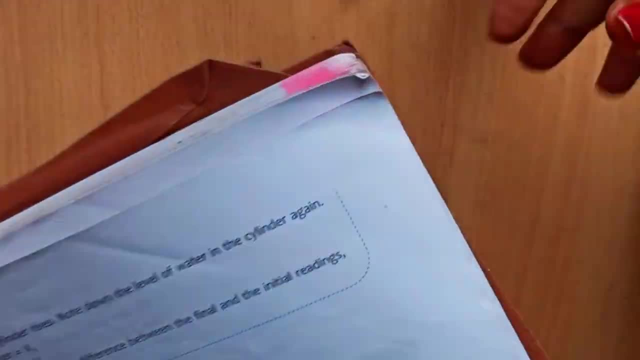 Final. wala ho gaya Sixty minus fifty Matlab ten Tika Kitna ho gaya Ten ho gaya Toh jo hum loong ko yaha par ten mila. Hum loong ko yaha par jo ten mila. 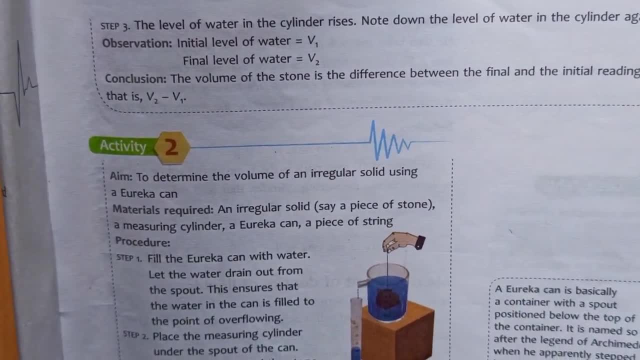 Wo ho gaya volume uss pathar ka? Bohot simple hai. Uske baad hum loong agar pustaya ek density nikaalo, Toh volume mil gaya. Mass de diya rehega Matlab, itna toh nahi puchega. 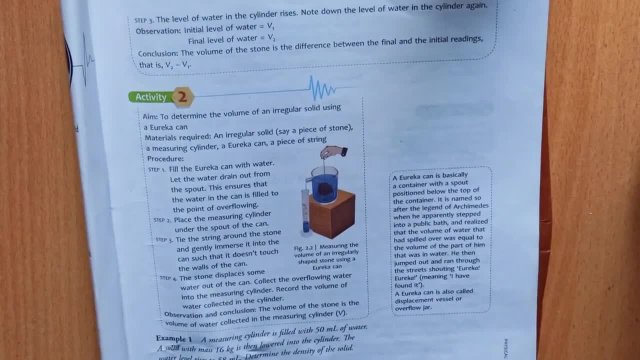 But main bataa diri ho, Aise aap loong volume nikaaloge, Ek dam easy tarika se Volume araam. se aap loong nikaal sakte ho, Tika Volume, kaise nikaaloge aap loong ko pata chal gaya. 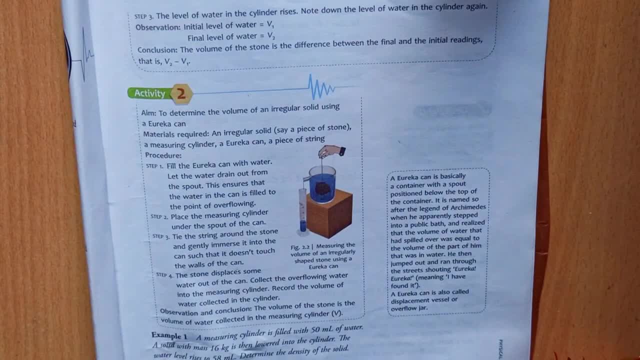 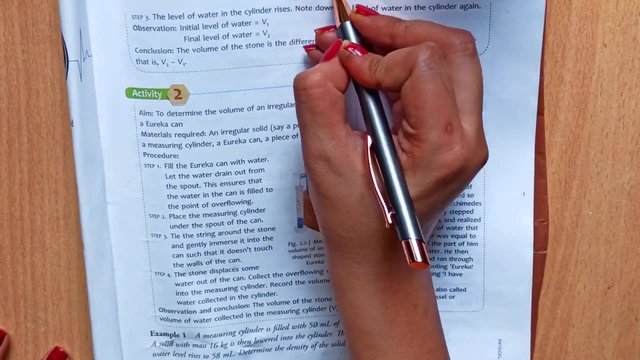 If question me Ya, fir aapki teacher aapko bolte hain, Ki aap batao iska density kya hoga. Toh bachcho, Density ka formula hota hai: Mass by volume. Aap loong ko volume mil gaya. 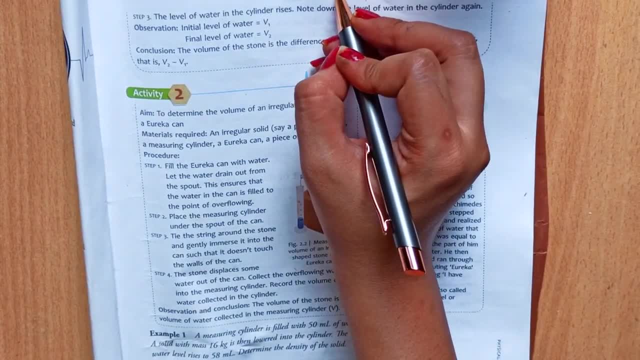 Jaisi ki ten mil gaya Aur mass question me diya: rehega Ki pathar ka mass suppose Suppose Suppose 20 gram hai. Jo bhi hai, Bust cancel out kar dina Jaisi ki aap loong mass me karte ho. 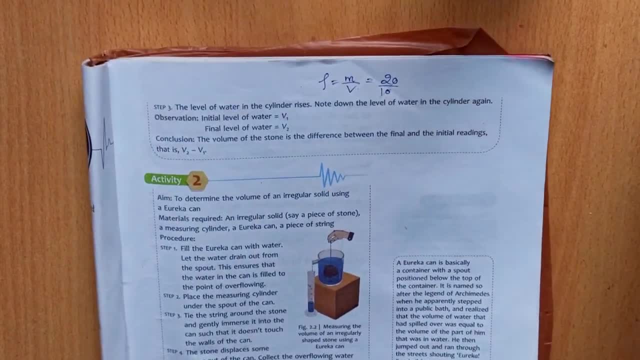 Bust Answer aajayega. Aap loong ko me itna pata hindi raha hai. Chalo Yaha wapis bata deti ho. Jaisi ki bachcho, Aap loong yaha dekho. 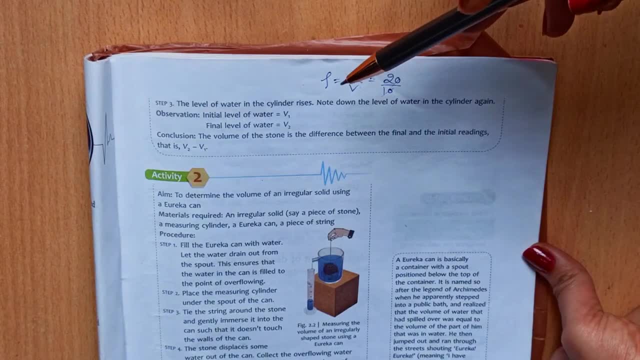 Suppose Volume Nikalane ke baad Density diya rehega Theek hai Aur density maangega Aapko teacher, aapko bushingi. Chalo, density batao, Agar mass diya hai. 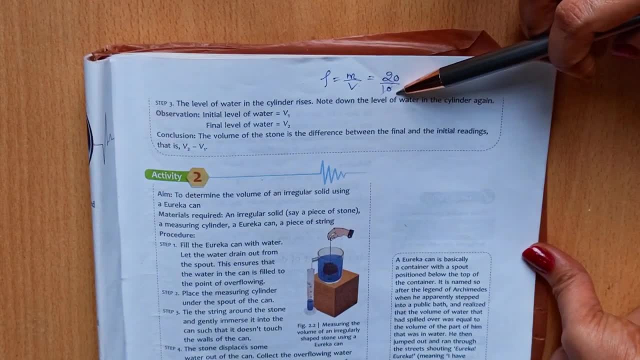 Toh formula: aap loong likhoge, Volume, aap loong nikal chukhe: 60 minus 50.. 10 aaya Aur mass pathar ka agar diya hai, That is 20 hai. Jo bhi diya rehega. 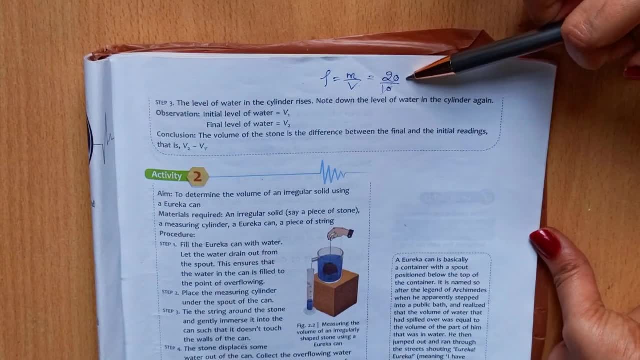 Bust Formula likke Values aap loong daloge, Solve karoge, And bust Aap loong, ko answer mil jayega. Yeh bhot simple hota hai Toh measuring cylinder ke saath kaam karna. 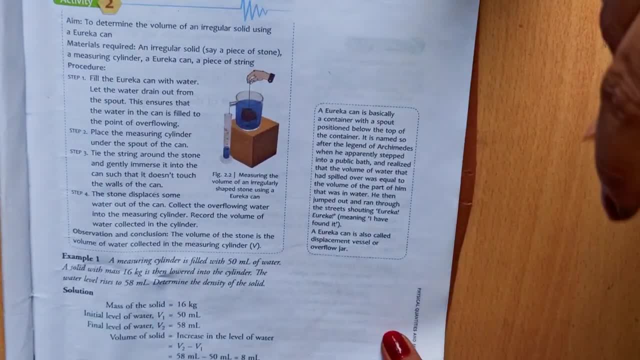 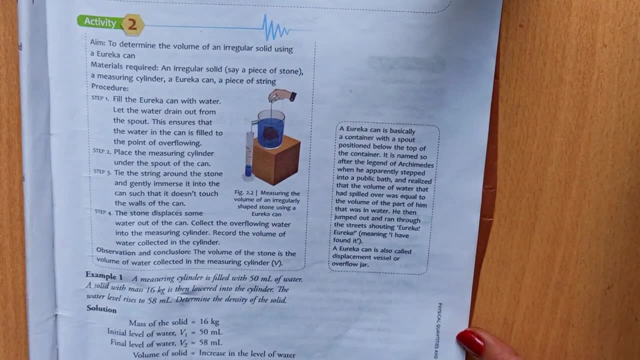 Very simple, Bhot simple. hai Aise koi tam sham nahi hai, Bhot, aise koi difficult ya critical saa cheez wo nahi hai. Abhi same irregular, solid hai Aur hum logo ko again volume nikalna hai. 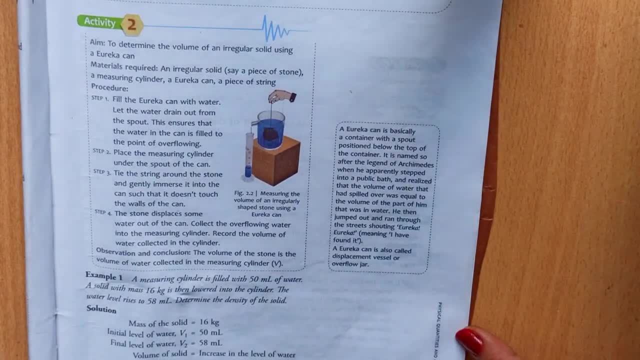 Lekin ya measuring cylinder ko use nahi karengi, Hum loong kis ko use karengi, Eureka can ko. So eureka can ko jis type se dikta hai: Bust yaha par hum loong ek beaker, ya fir jo bhi. 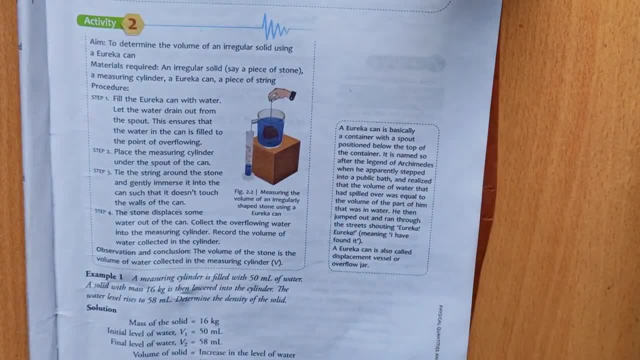 Ya, beaker toh nahi hai. Yaha par jis type ke kuch test yu. Ya fir apno measuring cylinder hi laga lo, Jis me scaling type ho Cheek hai. Ab dekho, yaha par kya diya hai. 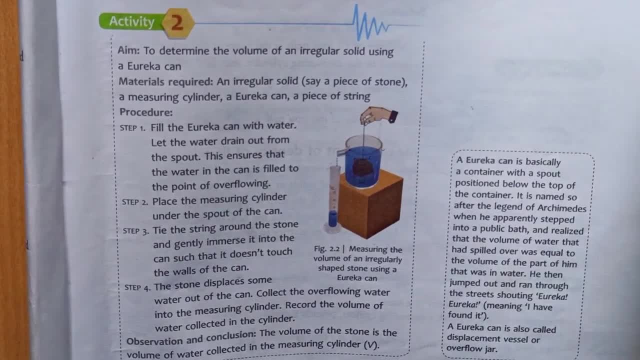 Dekho bachho. second activity me Hum loong ko same cheez karna, Irregular solid ka volume nikalna hai, Lekin yaha par measuring cylinder se nahi, Eureka can se hum loong ko use karna hai. 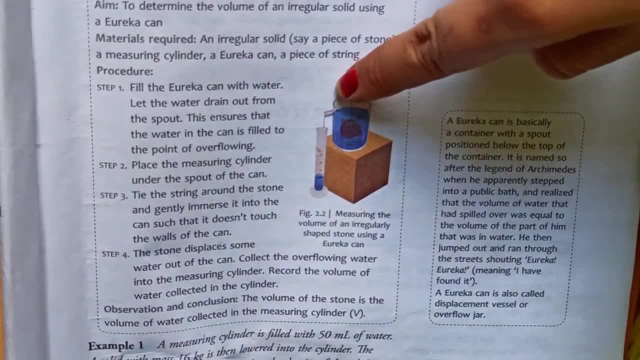 Like volume nikalna hai. So eureka, can, bachho, jis type se dikta hai. Ab loong, kis type se beaker dikha raha hai na Beaker ke side me na se spout hota hai, Tika, yaha par. 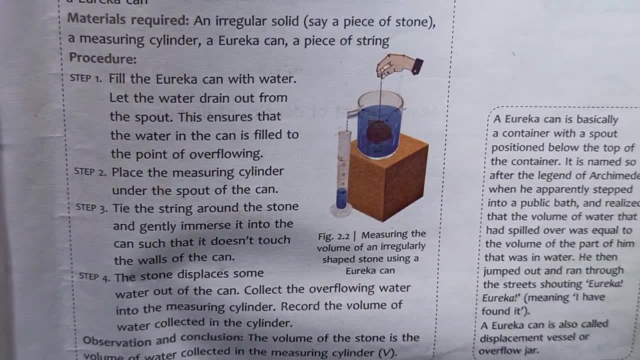 Ab loong ko toh dekhe, pata chal gaya hoga, Aur ab loong ke book me Ab loong ko aur clear diagram dikta hoga. Tika Toh hum loong ko sabse pehle kya karna hai, yaha par. 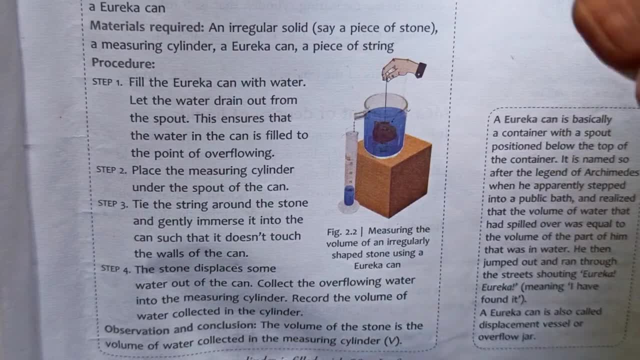 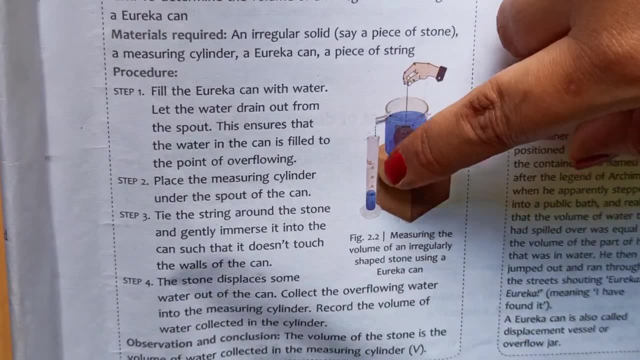 Kya kya samaan chahiye. Materials required: Kya kya chahiye? Aise eureka can chahiye, Mehliye the stone chahiye Irregular, solid, Aur ek measuring cylinder chahiye. 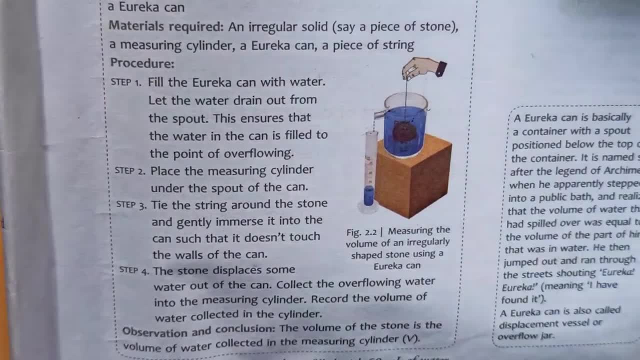 Tika measuring cylinder kyu chahiye Bataungi abko aage Tika na Acha Sabse pehle hum loong ko kya karna Ye eureka can e na Usko ab loong. 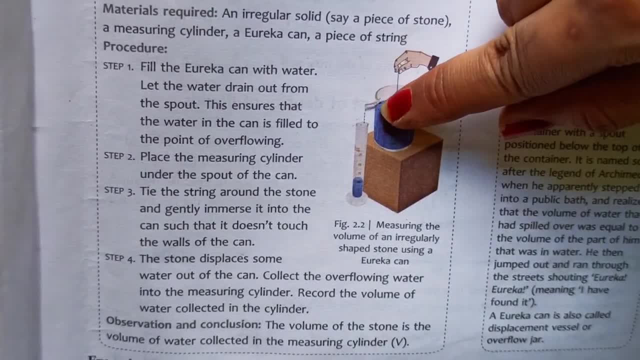 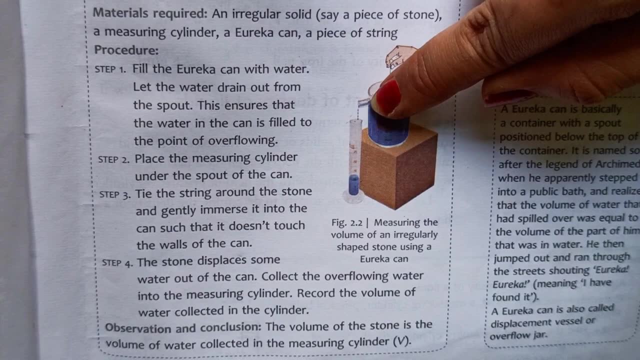 Pur achche se pani se fill kar do. Ab achche se matlab Ye point tak Aisa ki bas pani jisiki overflow ho sakhi, yaha tak Overflow karna nahi hai. Is point tak bhar do pani ki. 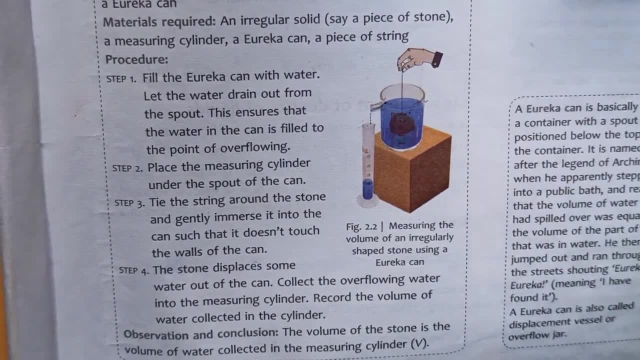 Aisa lagi ka ki ha Ab thoda sa. agar aur extra dale, Toh over flow shayad ho jaye Toh upar tak Spout, tak Ab loong ko Pura pani ko bhar dena hai. 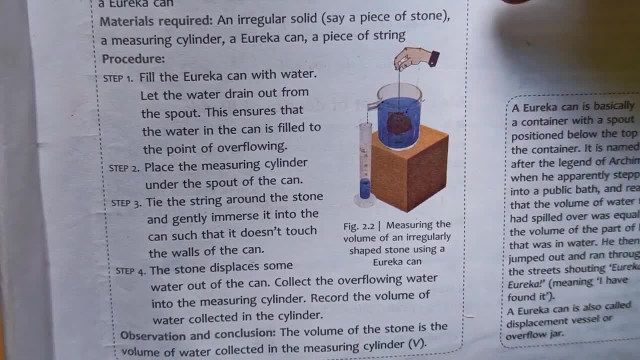 Uske baad Niche me set kar lo Measuring cylinder. Tik hai Uske baad Bachcho Ab loong, Dheere, dheere. kya karo Isko Achche se immerse kar vao. 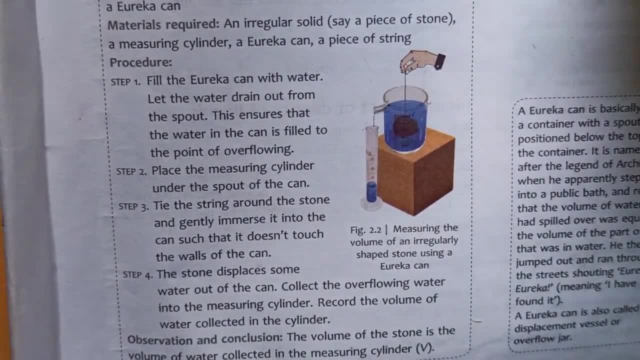 Aur is tarike se kar vao Ki Pathar. jo hai Wo side me like Touch na ho Tik hai, Jab ab loong Pathar ko dheere dheere immerse kar vaoge na, Toh ab loong dekhoge. 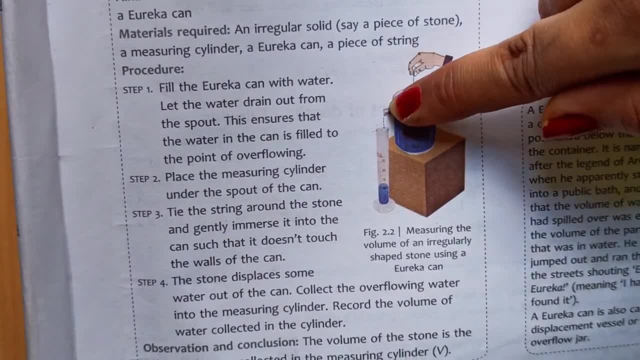 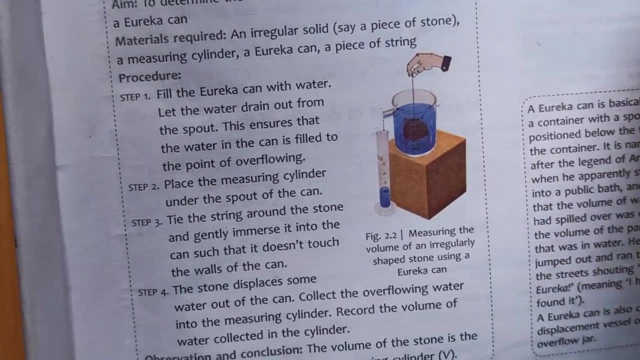 Ki yaha se jo pani Jo ab loong Upar tak pura pack kye the Ab wo over flow karega Wo spout se niche girega, Aur niche girega, Kahan girega wo. 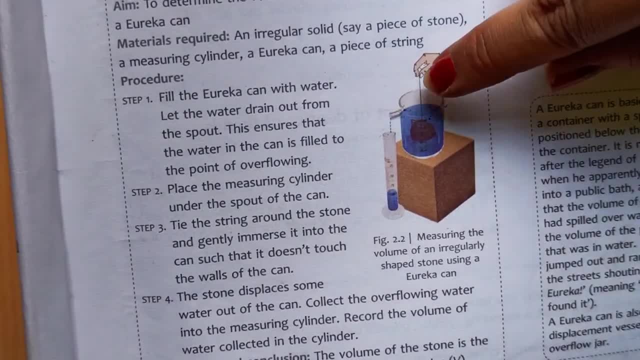 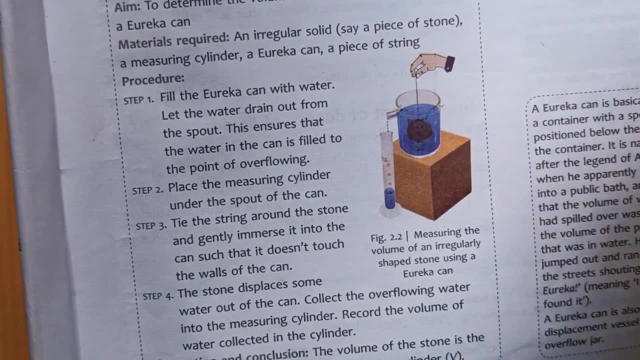 Measuring cylinder me Tik hai. Ab Ye jo stone jo andar jaa raha hai. Ye Kuch jaga lega Jo ye jaga lega, Toh pani upar ki taraf aega Tik hai. 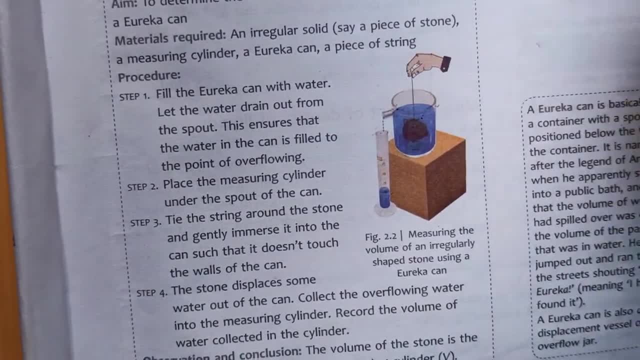 Kuki stone jo hai, Wo pani ko displace, karega Pani ke andar, wo jaga lega, Ab pani upar ki taraf uthega. Wo pani bahar girega, Toh, wo pani jitna bahar gira. 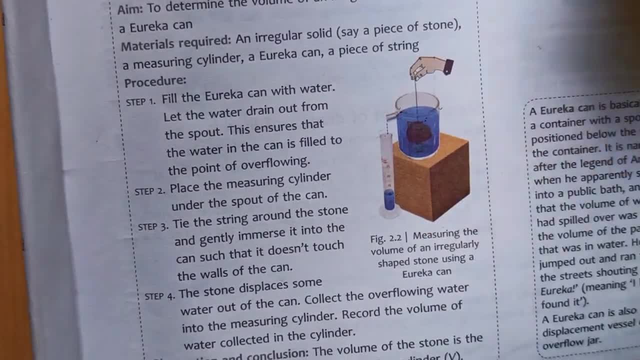 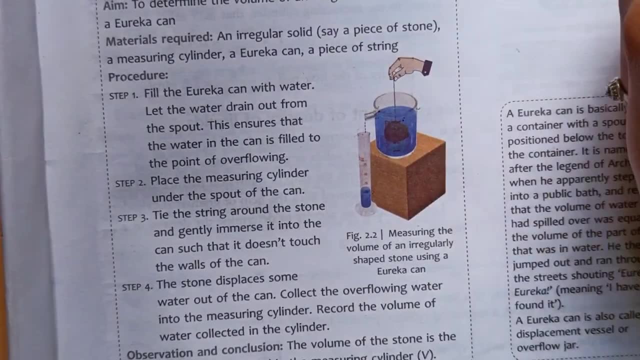 Usko ham loo measure kar lenge Kis me measuring cylinder. me Wo measuring cylinder ham loo ko volume de dega. Kuki measuring cylinder se ham loo ko aram se volume mil jata hai Wo measuring cylinder ham loo ko volume de dega. 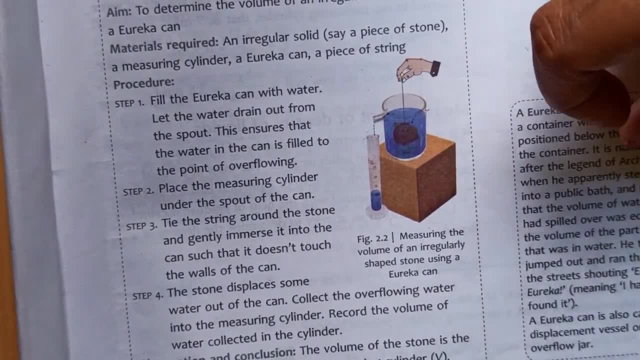 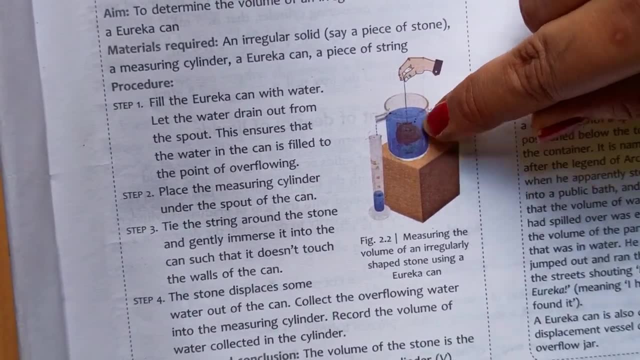 Kis ka Stone ka Aur bahut easily ham loo uss irregular solid ka volume jaan payenge, Toh yaha par jitna pani girega na. That is equal to the volume of this irregular solid. Bahut easy hai bachoi. 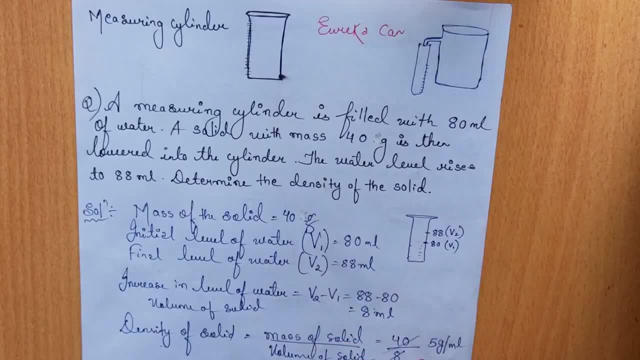 Kaafi easy, hai, Kaafi easy. I hope ap loo ko samajhme toh aya hoga. Ek numericals kar lete hain. Iss se related Measuring cylinder related. Bohut simple hai, Question me diya hai. 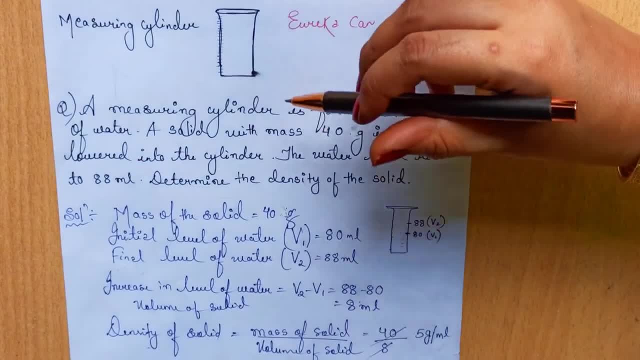 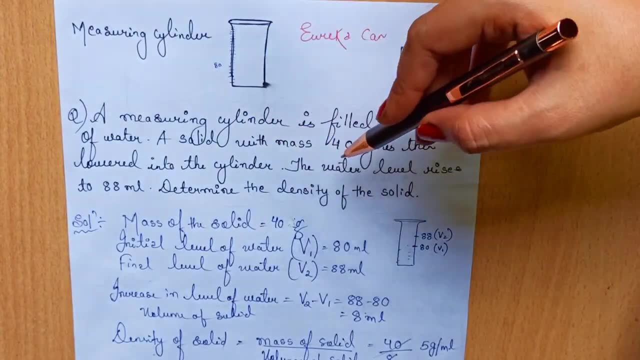 A measuring cylinder is filled with 80 ml of water. Jisi ki ye measuring cylinder Yahi deklo Suppose ye 80 ml pani. se bharti Suppose yaha 80 ml pani hai A solid with mass 40 gram. 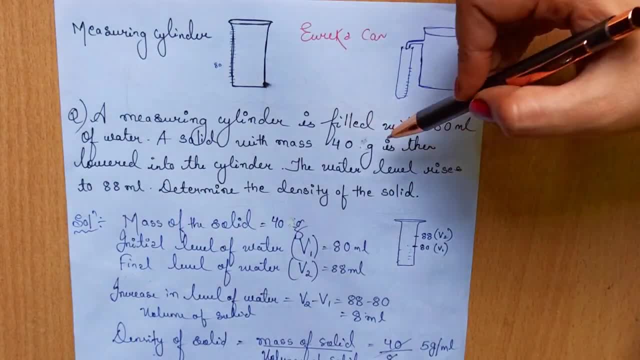 Ek solid hai, jiska wajan hai 40 gram Ji ka matlai hota hai. gram Is then lowered into the cylinder 40 gram ka pathar ko hai Main pathar bol rahe ho. Solid me kuch bhi ho sakta hai. 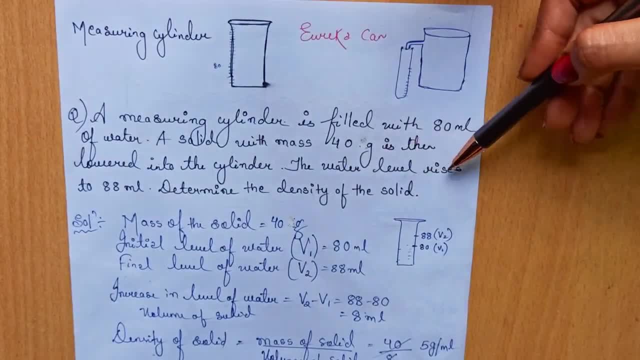 Usko ham loo pani ke andar me yaha par immerse kar waha hai Toh water level badke 88 ho gaya Pahle 80 tha Original, Aur badke wo ho gaya 88.. 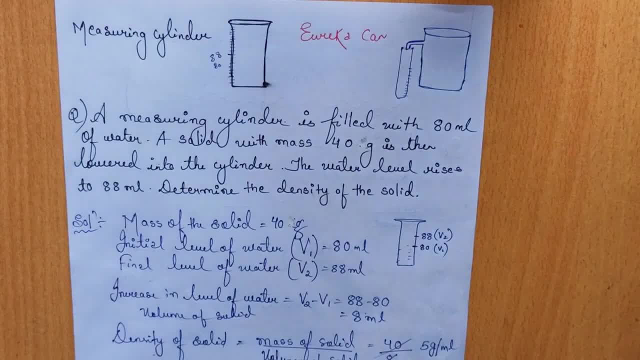 Suppose yaha 88 ho gaya Thik hai Hitna ho gaya 88. Ekdum simple hai. Ab bol raha hai Density nikal ho. Kya nikal ho Density Thik hai Density nikal lenge. 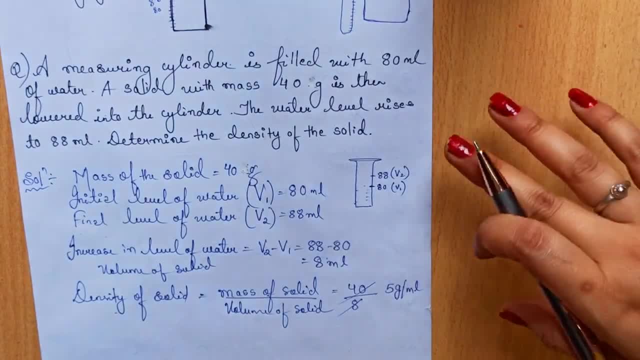 Density nikal lenge bol raha hai. Toh sabse pehle density ka formula kya hota hai. Main bachu ekdum simple tarike se bata rahe ho: Dekho, ye toh book ka tam cham tha. 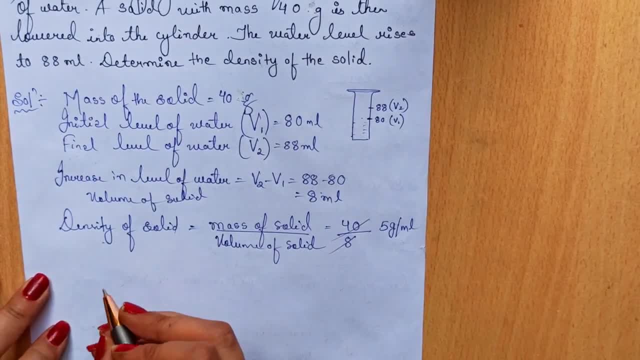 Toh mai leak di thi Ekdum simple tarike se bata rahe ho. Dekho density ka formula kya hota hai: Mass by volume. Mass diya hai pathar ka, Kitna diya hai 40 gram. 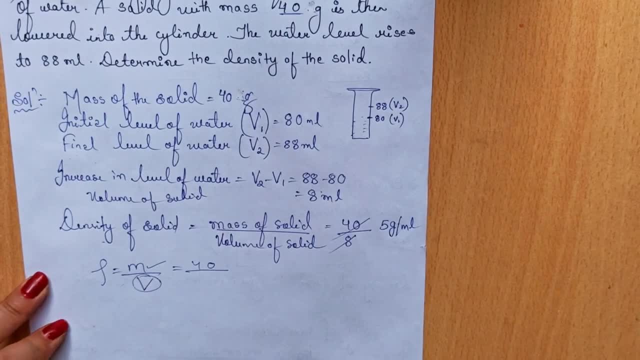 Toh yaha, toh chalo, a jayega 40 gram, Lekin volume is solid ka kitna hai. Wo toh amko pata hi nahi hai Book, kya question me kahi par likha hai, ki solid ka volume kitna hai. 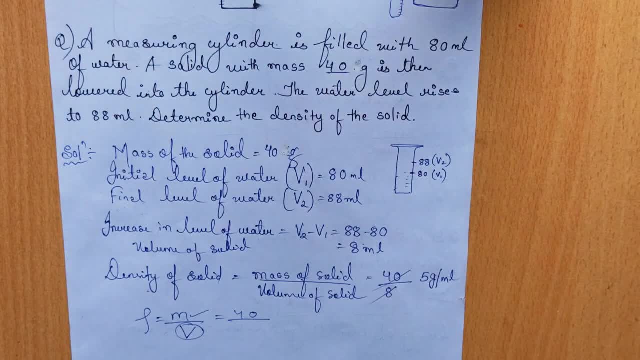 Kahi par bhi ni likha hai, Par measuring cylinder ke andar me pani tha. Ham loko pathar dalna hai, Solid dalna hai, Pani ka level bar raha hai. Toh waha amlo pade hai. 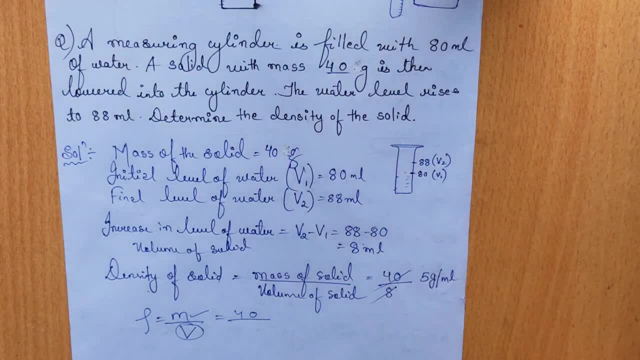 Aage me amlo pade hai, ki wese amlo volume calculate kar sakte hai. Pehle 80 tha, Phir 88 hua. Toh volume kese nikalte hai. Final matter is original 8 ho gaya. 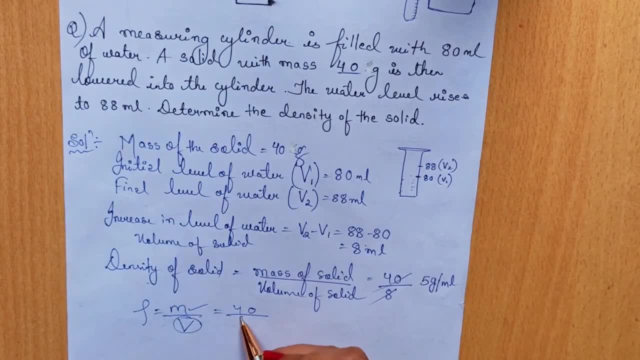 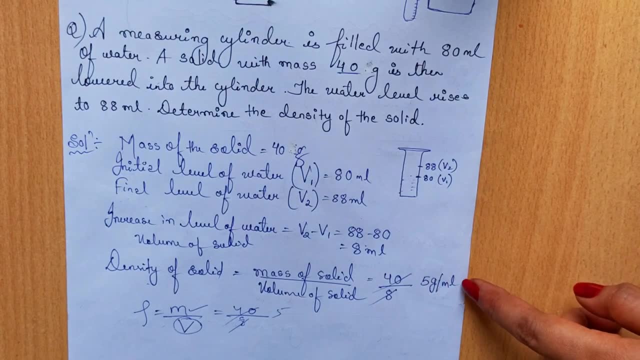 Toh 40 by 8.. 40 by 8. kar dete hai Usko kato 8 by 5 ja 40.. Aage answer Toh 40.. 5. g by ml. Ab ye g by ml kahan se aya.